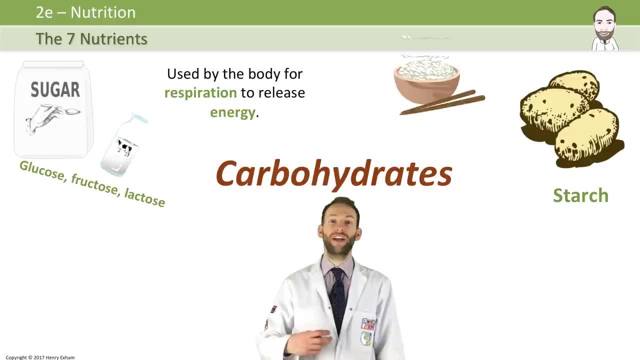 if you know about the respiration equation, you'll know it's glucose plus oxygen goes to carbon dioxide, plus water, plus energy. So the glucose you need for that reaction comes from our carbohydrates. But if you have too much carbohydrates, too much energy, then 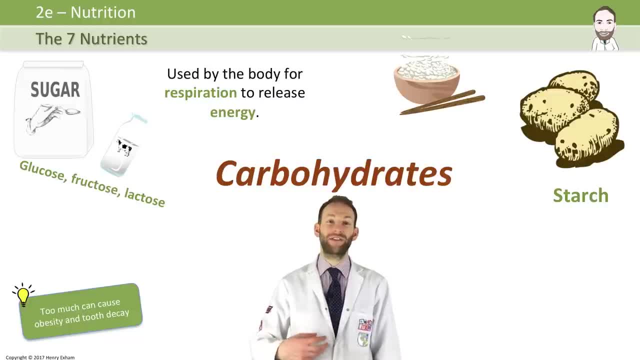 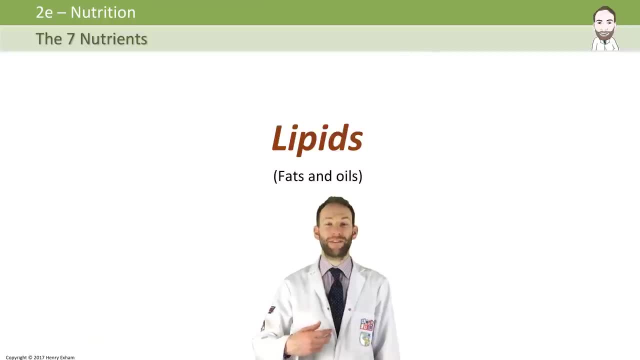 your body decides to store that as fat and it can give you obesity or it could cause tooth decay. Now, lipids is the proper name for fats and oils. Food high in animal fats includes meat, butter, cheese, milk, eggs and oily fish, And foods high in plant oils include olive. 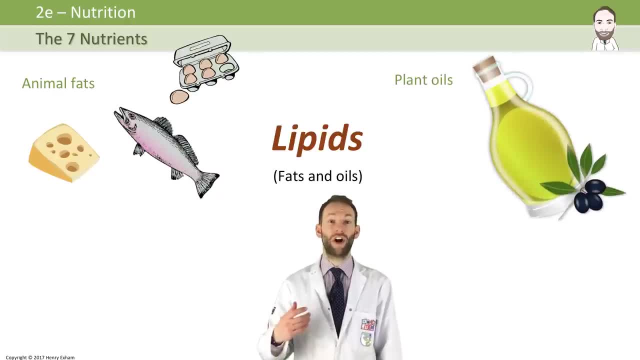 oil, sunflower oil, rapeseed oil and margarine. On the whole, lipids from animals, which tend to be saturated fats, are worse for you than the unsaturated fats you get from plant oils. Now what do we use fat for? Fat has quite a bad name, but actually we need fat in our 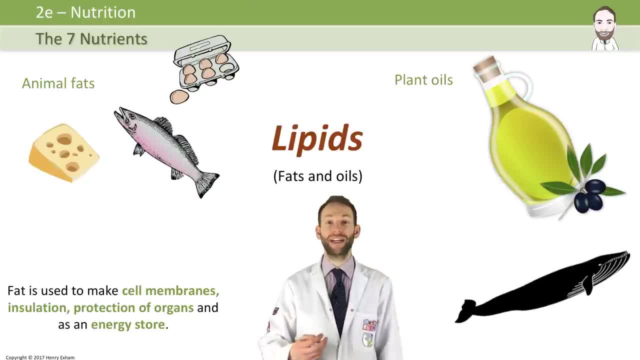 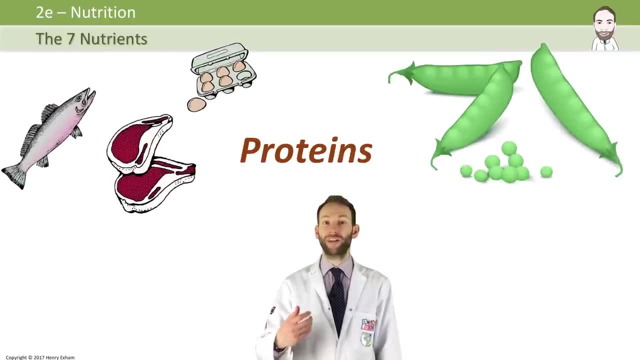 diet. We don't need too much of it. It's very important for making cell membranes, for insulation, for protection of organs and as a store of energy. Proteins, Now animal foods high in protein include meat, fish, cheese and eggs. You can. 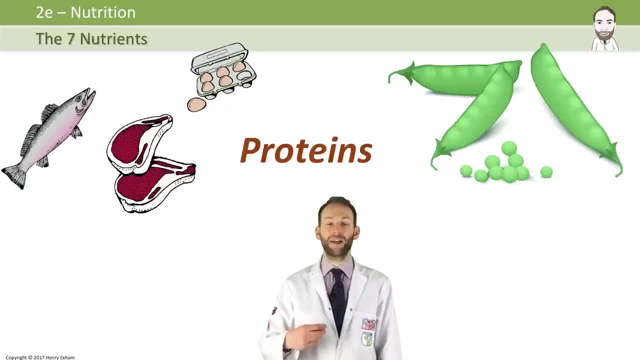 get protein from plants- things like beans, peas and nuts- But meat is a primary source of protein. It's a better source of protein. And what do we need it for? We need it for growth and repair of tissues, Replacing cells. 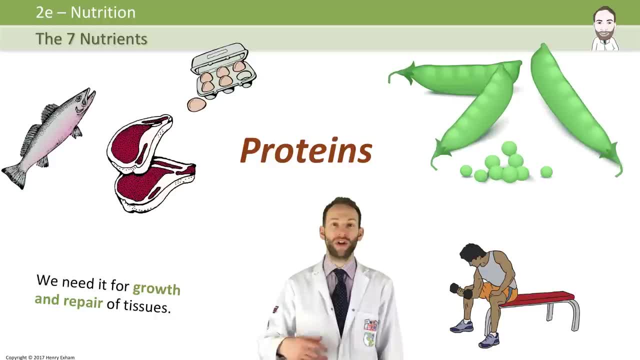 Very important. when you're growing, either as a baby or an adolescent, And also even when you stop growing, you need to replace cells constantly, every day, And we need protein in order to do that. Vitamins. So there's a couple of vitamins you need to know about: Vitamin A, which is 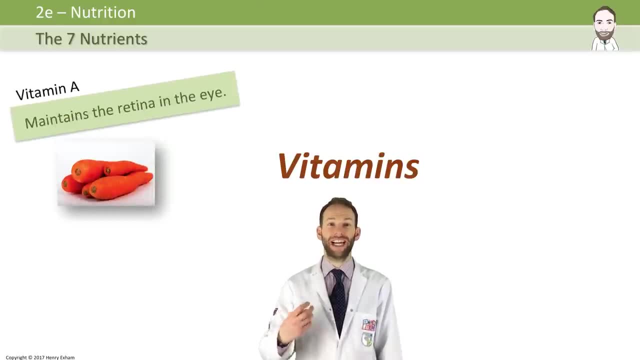 used to maintain the retina in your eye, And you get that from carrots, fish, liver oils, liver butter and margarine. So that old wives tale of carrots helping you see in the dark, There's actually a bit of truth to that, because they're high in vitamin A, which is used to 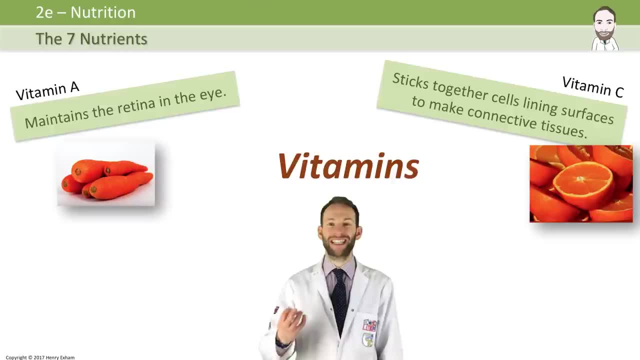 help build your retina, Vitamin C, which is used to sort of stick cells together, lining surfaces, to make stuff we call connective tissues, and it's found in fruit and vegetables, especially citrus fruits. And if you don't get enough vitamin C it can cause scurvy, where your fingernails will start to bleed. 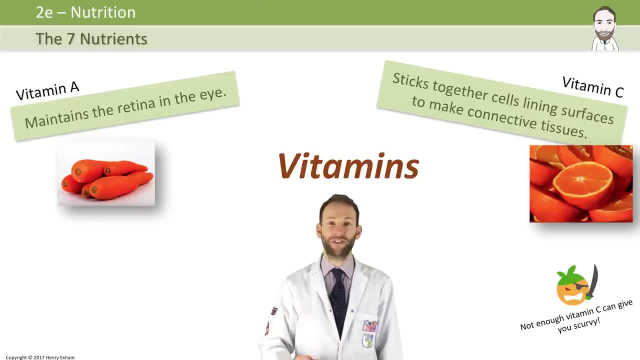 and bleeding gums. Very famously, pirates always got scurvy because if you went on long voyages, you could never take any fresh fruit and veg with you. even though you could take animals to slaughter and carbohydrates, you couldn't get vitamin C. 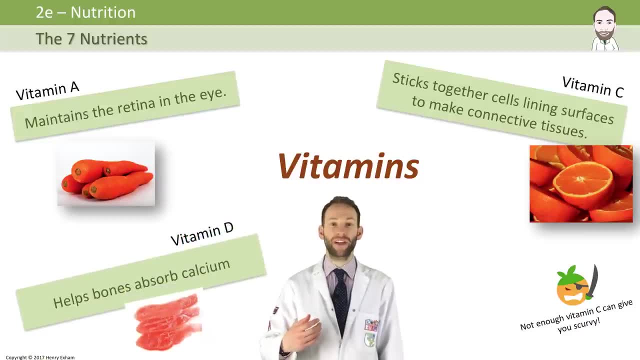 And lastly, vitamin D, which helps bones absorb calcium, And you get that from things like fish, dipper oils again, and also from dairy products, But it's also made in your skin when you're exposed to sunlight. What about minerals? So there's two major minerals, really, that you need to know about. 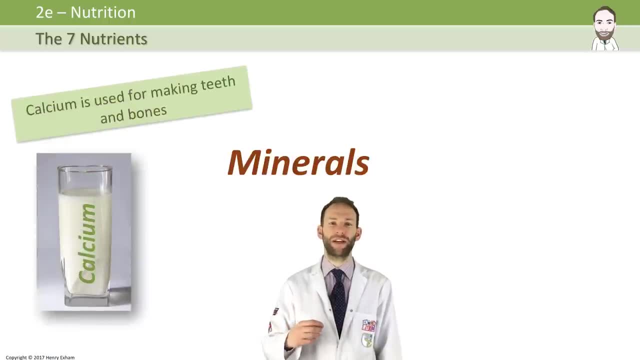 but a lot of these minerals are the same elements you would find on a periodic table. What about calcium? We're going to look at calcium, which is used for making teeth and bones, very high in dairy products and fish and bread and some vegetables. And if you don't get, 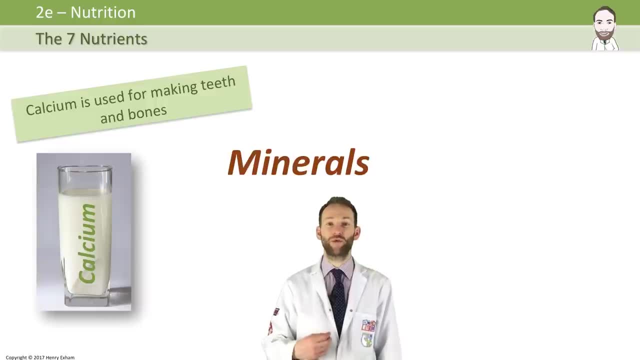 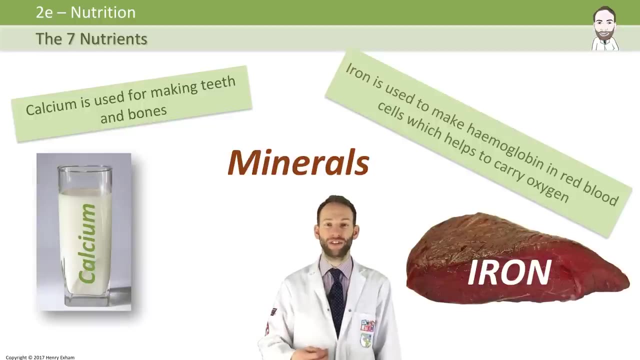 enough calcium, then your bones won't develop properly and you can have a disease called rickets. And iron, which is used to make haemoglobin in your red blood cells so that they can carry oxygen, So very important, And you get that from things like red meat, liver, eggs. 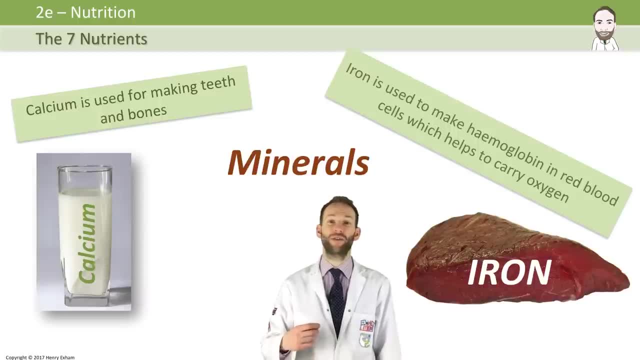 and some vegetables like spinach. If you don't get enough iron, you can end up with a disease called anaemia. What is anemia? Well, people don't think water is a nutrient, but it is, and it's included in these seven. 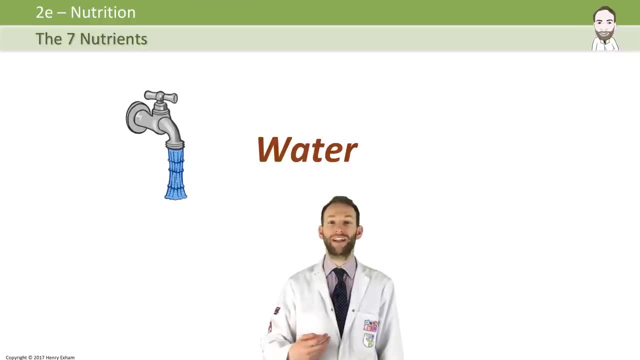 nutrients, and it's very, very important We need it obviously to stay hydrated. What that means really is to make sure that osmosis works properly between our cells and our blood and our tissue fluid. We don't want our cells to shrivel up if they don't get enough water. 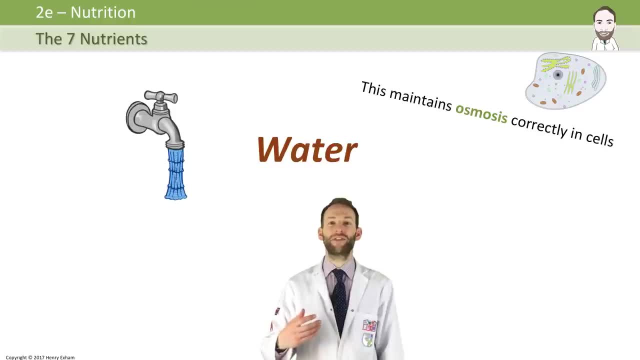 but equally we don't want our blood pressure to get too high if we have too much, So it's very important that water levels are maintained, Also because it's our blood plasma. a lot of reactions take place there and we use it. 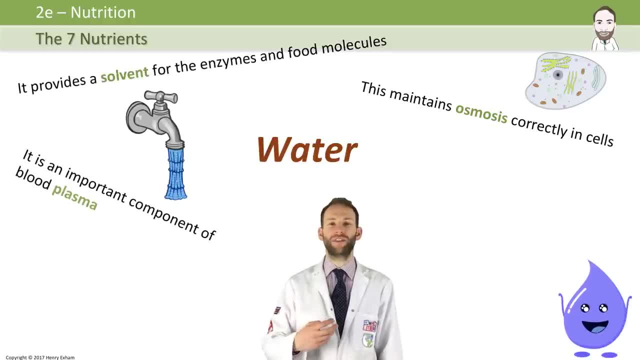 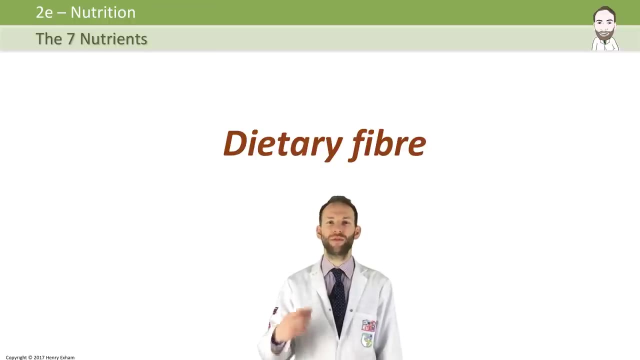 around our body, So it's very, very important. You need to drink about between 1.5 and 2 liters of water a day. The last nutrient you need to know about is fiber. Now, dietary fiber isn't actually something that you digest and absorb, but it's very, very important for maintaining what we call. 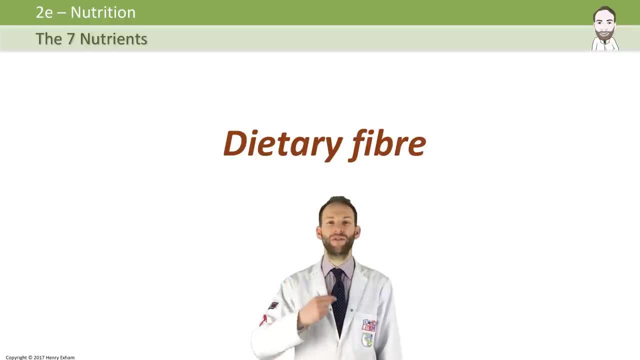 digestive transit. Your food needs to pass through the digestive system from your mouth to your anus And along that It's to help it sort of Along that journey. we need the fiber Now you get it from mostly cellulose that's found. 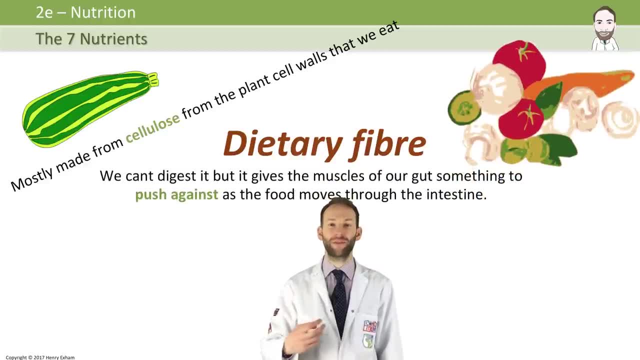 in plant cell walls that we eat. So fruit and vegetables are very good sources of fiber And, like I said, it gives your gut something to push against, so that it moves the food through the digestive system. Now, if you have too much, though, then it will move too. 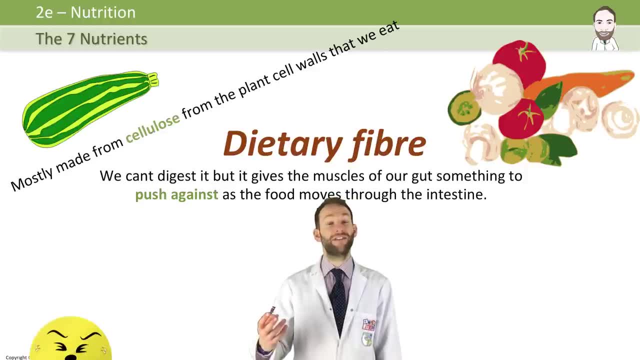 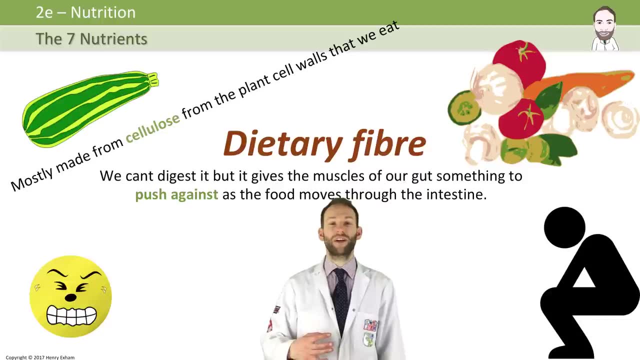 far through the digestive system and you can end up with diarrhea. And if you have too little then you can end up getting constipated because it won't move fast enough through the digestive system. Now you don't need all these seven nutrients in equal amounts. That wouldn't be a healthy 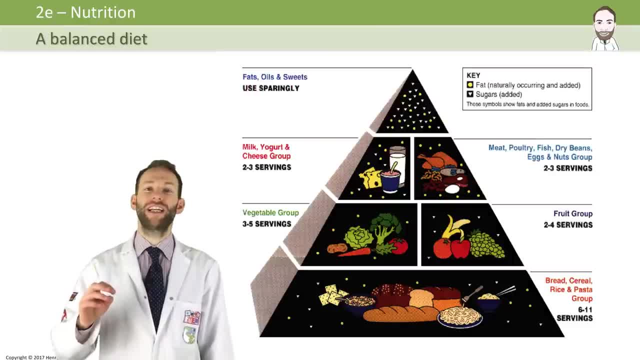 diet. A balanced diet has all the seven nutrients in the correct amounts. So this pyramid here is a bit of a representation of that. You have carbohydrates at the bottom there and then some fruit and vegetables, Next one protein, dairy- and some fats at the top. 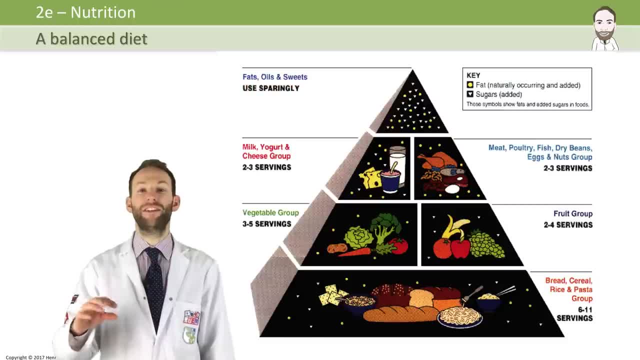 Realistically now we're thinking we actually need a lot more fruit and vegetables. even that's shown by this pyramid Um. People end up having too much dairy fats and protein and not enough of the fruit and vegetables underneath to maintain a healthy, balanced diet. But not everybody's diet is. 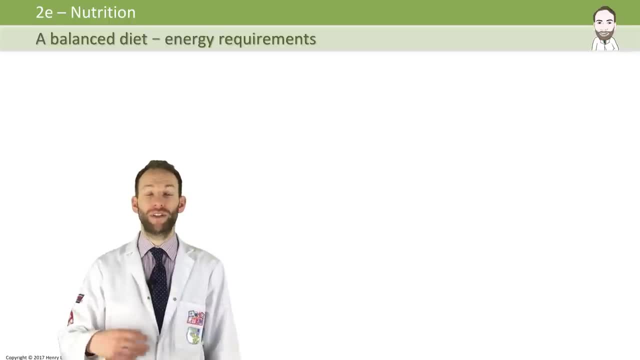 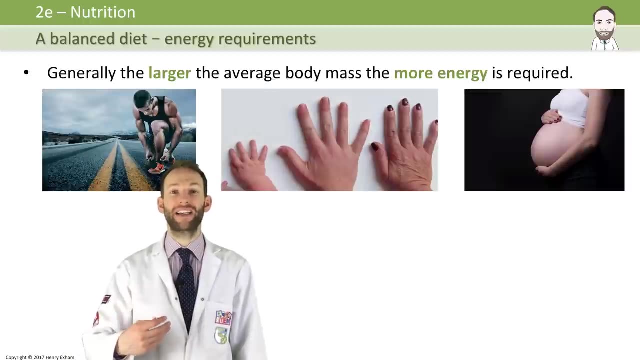 the same. Different people who have different jobs or different ages will potentially need different diets because they have different energy requirements. The larger the average body mass, the more energy is actually required. A two-year-old child only needs about 5,000 kilojoules a day, whereas a 15-year-old boy needs about 12,000 kilojoules a day. 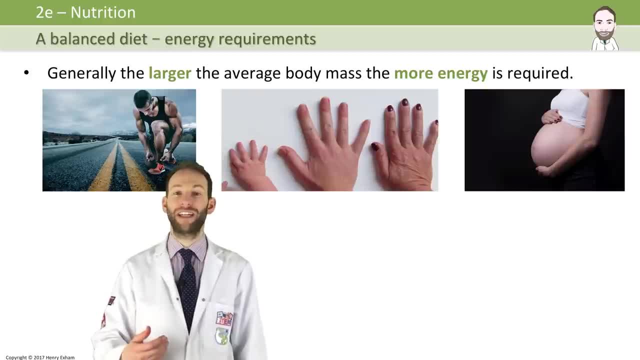 So people have different requirements. If you're an athlete, you're going to need to eat more food, more calories, to get more energy. If you're pregnant, you're going to need to eat more as well, not only because you're trying to feed a growing baby, but because 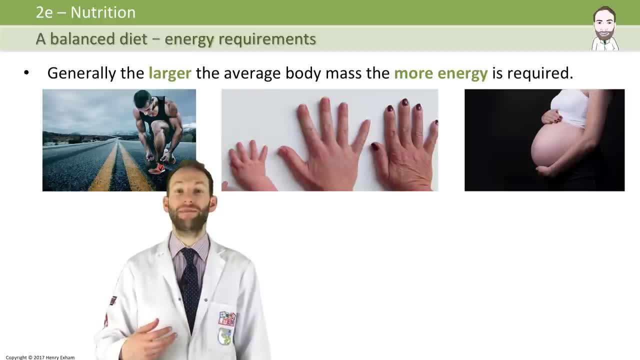 you are physically heavier and it takes more energy to move around on a daily basis, So you're going to use up more energy. A manual worker is going to need more energy per day than an office worker, So it's important to eat the diet that is right for your lifestyle. Subtitles by the Amaraorg community.